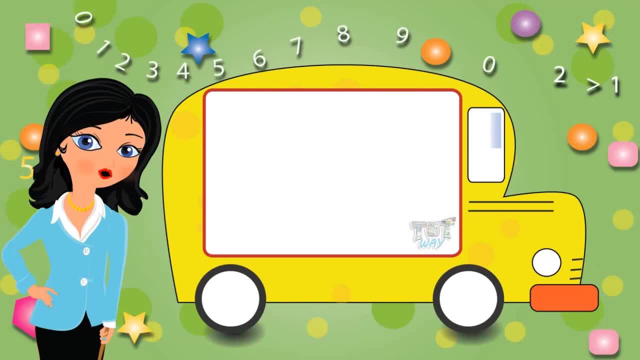 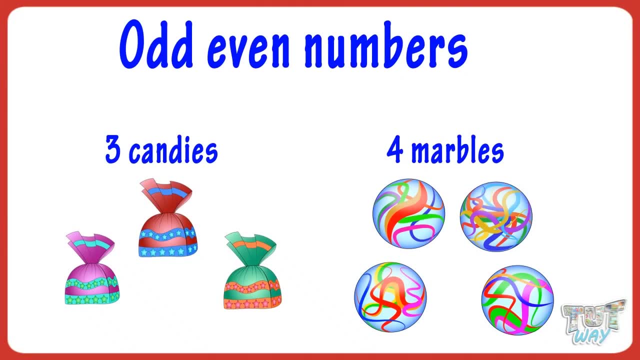 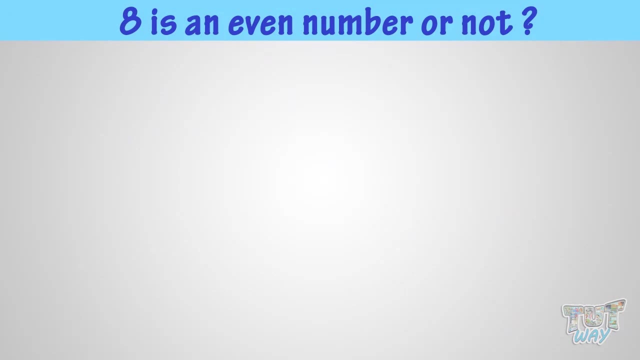 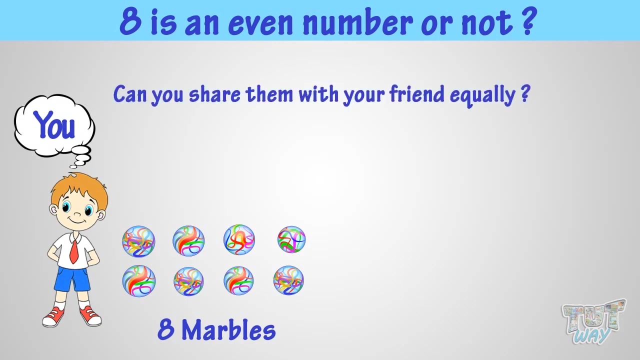 Hi kids, Today we will learn what are odd and even numbers. Let's start with even numbers. Let's see if 8 is an even number or not. You have 8 marbles. Can you share them with your friend equally? Let's see: Yeah, You can give 4 to your friend and keep 4 with you. 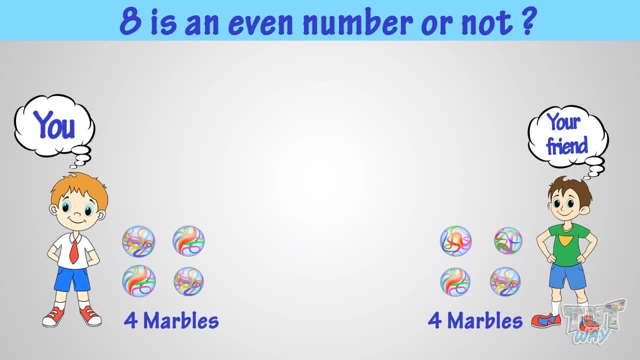 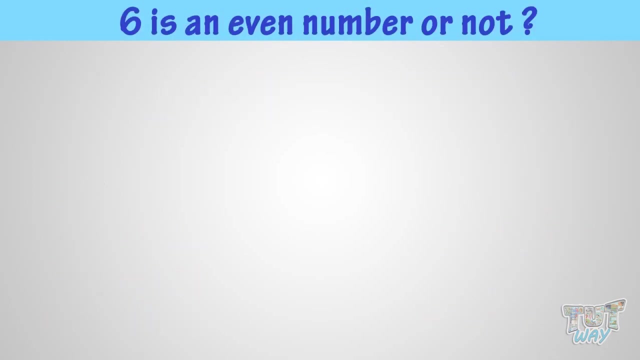 And any number of things that you can equally share between 2 are even numbers of things. So 8 is an even number, as we can share 8 things equally. Let's take another example. Let's see if 6 is an even number or not. You have 6 candies. 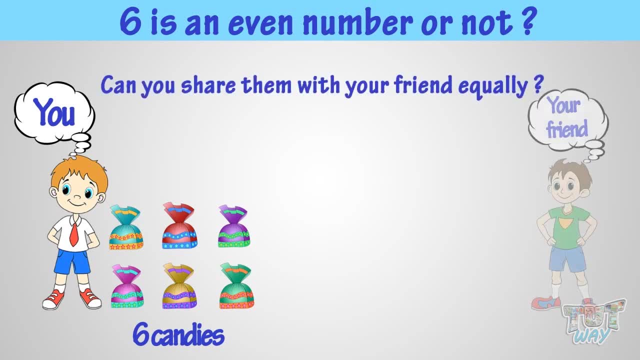 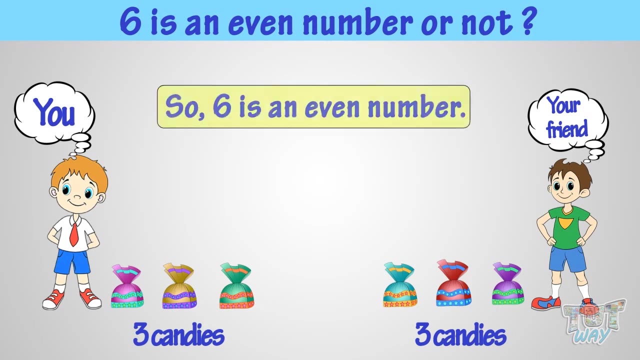 Can you share them with your friend? Let's see, Yeah, You can give 3 to your friend and keep 3 with you, And any number of things that you can equally share between 2 are even numbers of things. So 6 is an even number, as we can share 6 things equally. 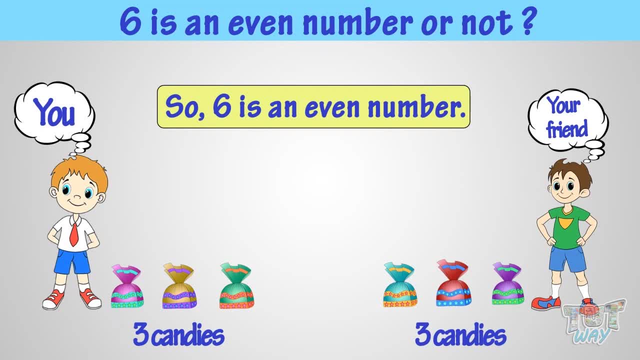 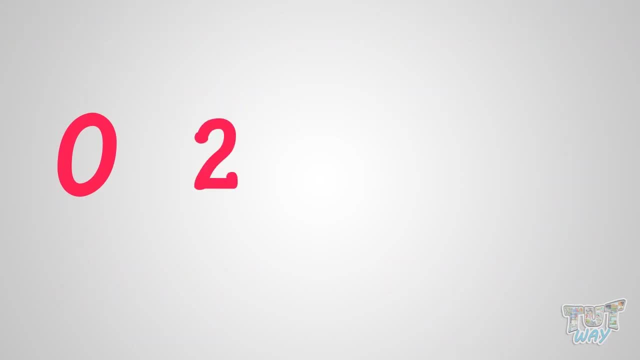 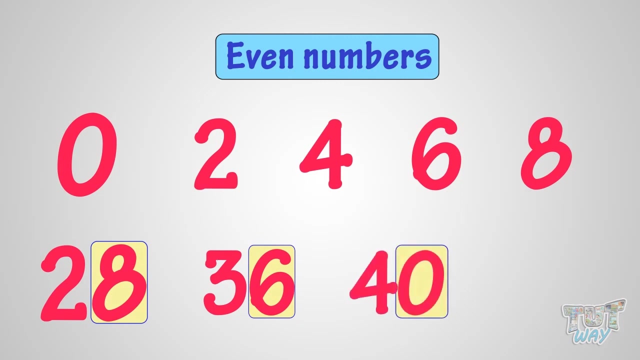 Wow, That's so easy. Also, don't forget: 0,, 2,, 4,, 6 and 8 are even number of things, and all the numbers ending with them, like 28,, 36,, 40 and 50, are even numbers. 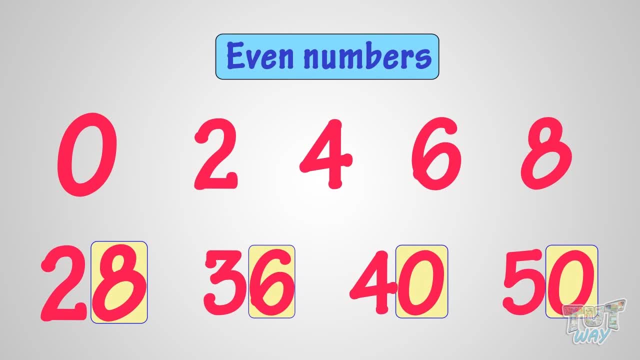 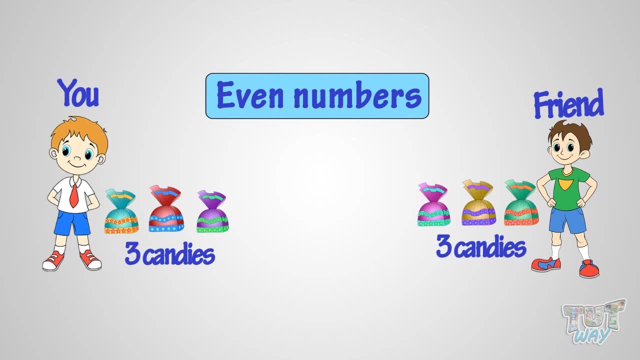 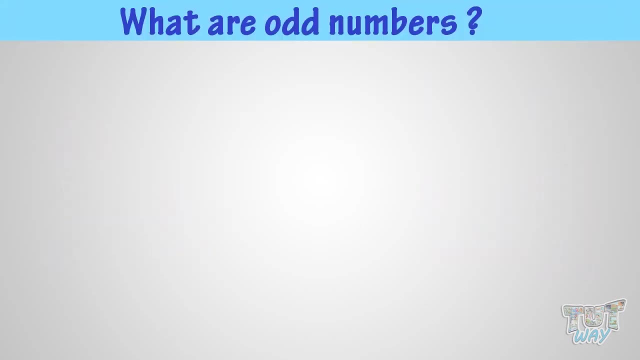 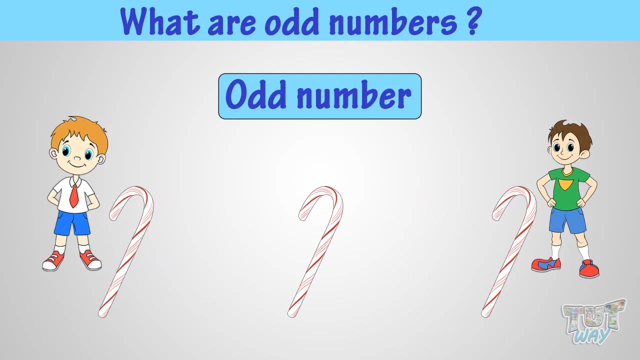 So what have we learned? We have learned that any number of things that can be shared equally are even numbers of things. Okay, now let's learn what are odd numbers. It's exactly the opposite of Even numbers, That is, if you cannot share a number of things equally between the two, they are odd number of things.